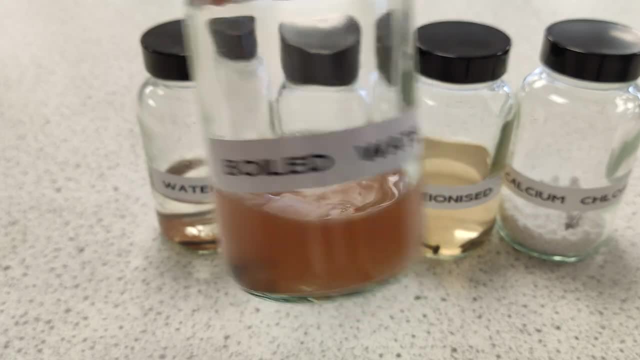 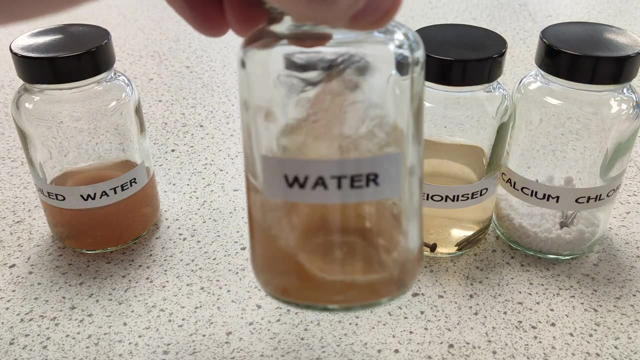 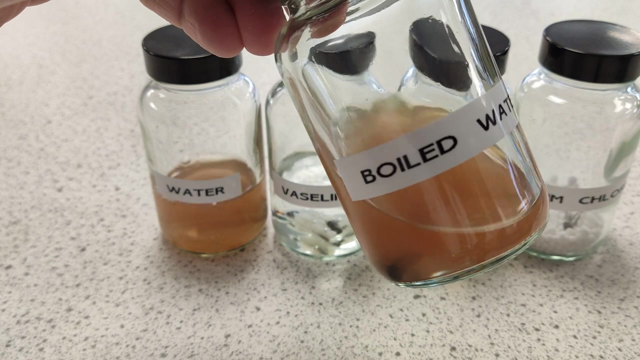 I can give it a shake and it looks pretty rusty, doesn't it? Standard water, there you go. So there's my standard water. Let's give it a little shake. That's definitely rusted. It's interesting because the bored water and the water, they're about the 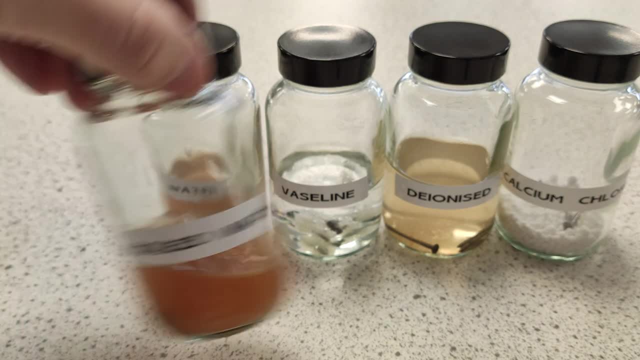 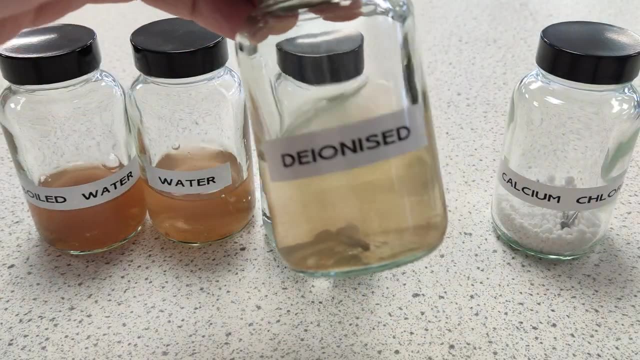 same actually. So even boiling it, I think the problem is that some of the oxygen and gases can dissolve back in. Let's pick out the deionized. I also thought I'd try deionized Now. this one is a little bit less rusty than the others. 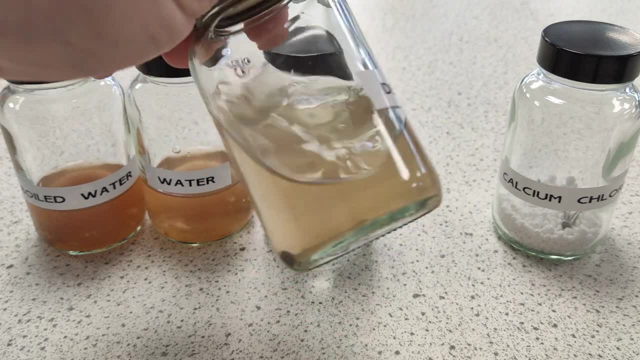 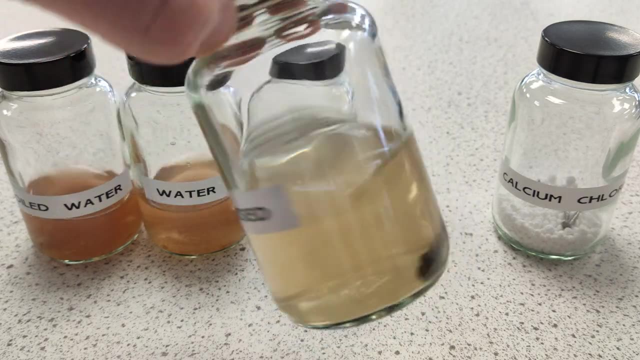 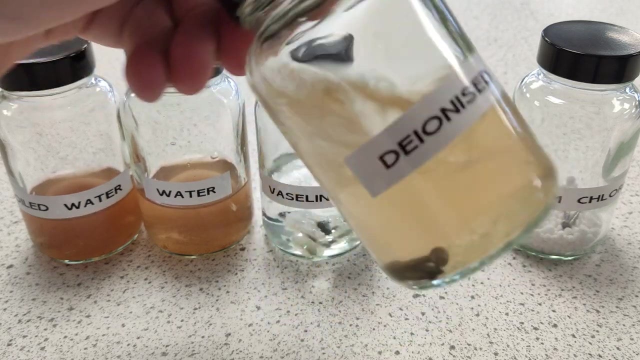 but part of that reason is because I started it off afterwards. I failed with the boiled water to make much progress, so I thought: well, let's give it a go with deionized. Do you know what? it still does it. It's got enough in there for it to be a problem because it's got iron oxygen. 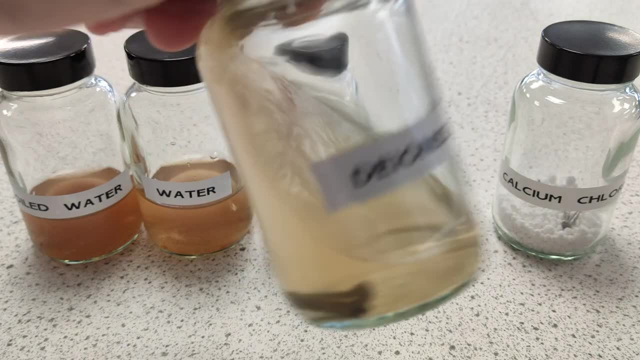 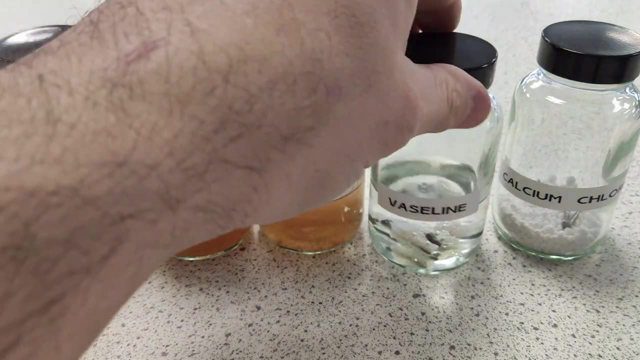 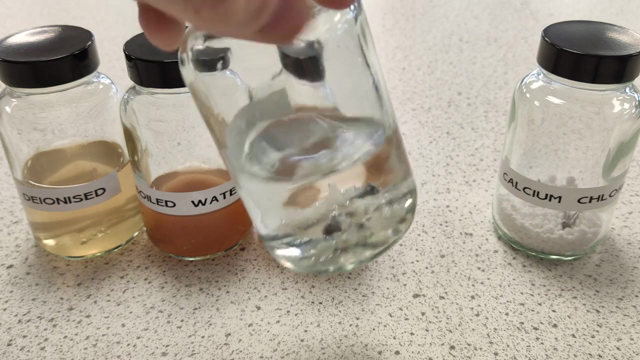 water. So it's not the ions in there that create the problem. it's the iron, the oxygen, the water combined, the fluidy ones to start with, and we've got one more. now. what have i done with this? well, it's real simple. we've just smeared some vaseline over the top of the nails. that's pretty good. i'm quite. 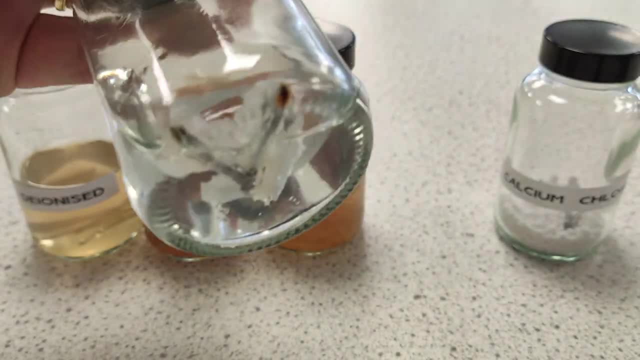 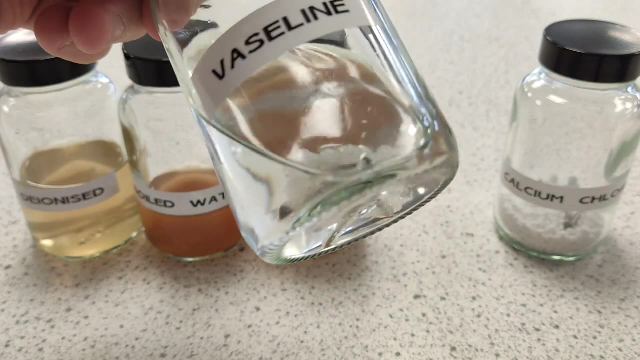 impressed with that. i will show you we failed slightly. look at the end there. where there's no vaseline, it has rusted so the vaseline can work. it's kind of like your car when you put a coating underneath your car and it slows the rusting down. so that's your underbody seal working. 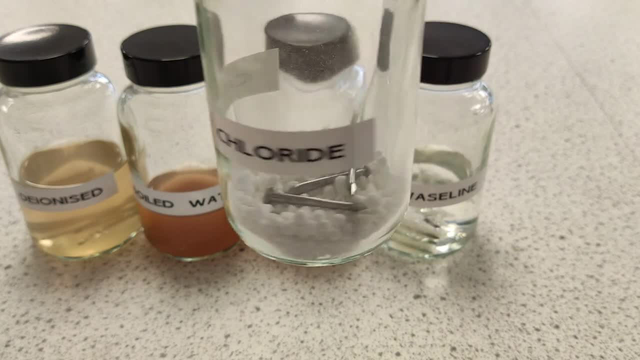 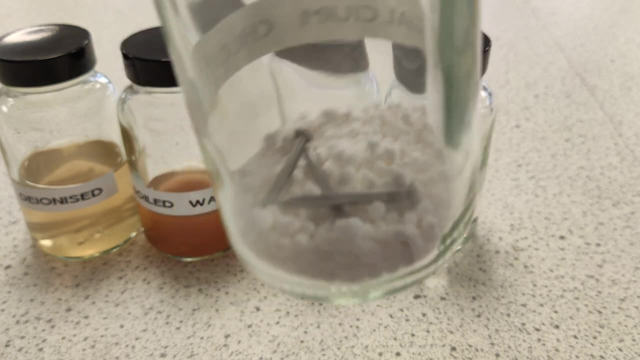 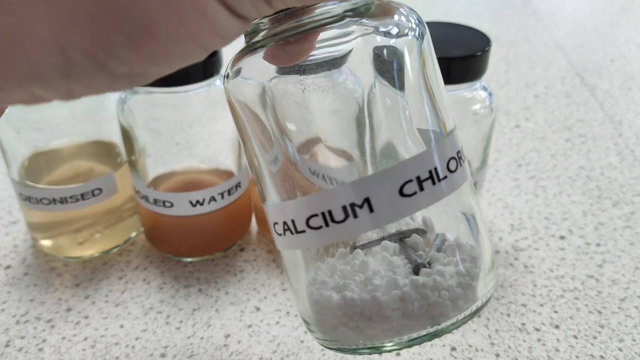 this one is the gem: calcium chloride. so look at my lovely nails. they're perfect. they're not rusted at all. so what we've done is we've dried them out. we've removed any chance of water being in there. there's oxygen there. no water means no rusting. so calcium chloride is the winner. and there we. have our little rusting experiment. if you like this video, please subscribe.